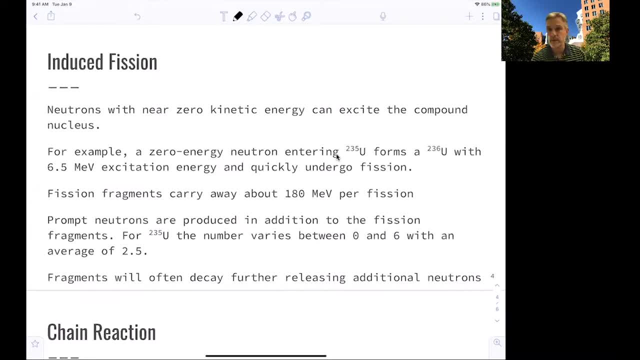 This forms uranium-236. And the fact that the neutron is being absorbed excites then this zero kinetic energy. neutron excite the daughter compound nucleus with an excitation energy, in this case of 6.5 MeV, And because of that it then quickly undergoes fission. 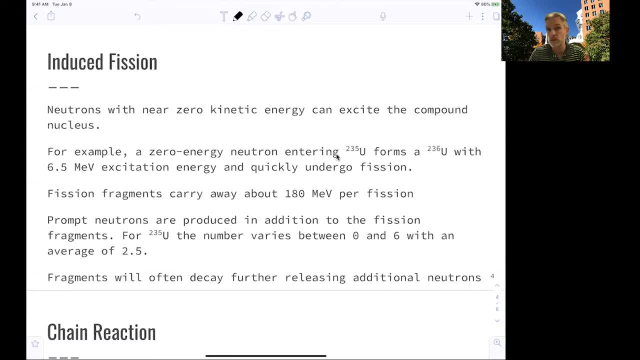 So you basically add a thermal or zero kinetic energy neutron And When it's being absorbed it immediately causes the fission process. The fission fragments then carry away some energy. In this example here it's about 180 MeV. 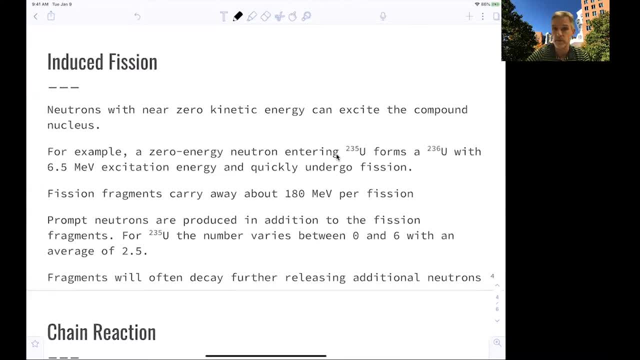 And additional prompt neutrons. And so those additional prompt neutrons, depending on the specific decay process, the number can be varying between 0 and 6.. And for uranium-235, the average number is 2.5.. And then the fragments. 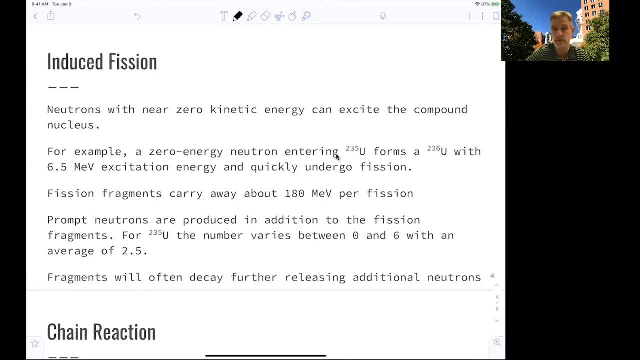 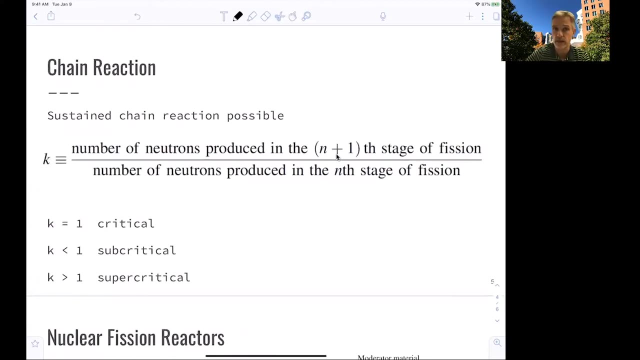 They might undergo additional decay process- maybe better decays, alpha decays- And when they do that, they can also release additional neutrons. So interesting now is to see whether or not there can be a self-sustained reaction, a chain reaction. 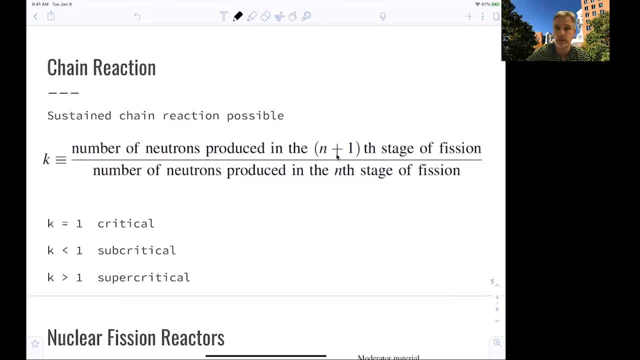 And whether or not this occurs depends on the number of neutrons being emitted. So if the number of neutrons produced in the n plus first stage of the fission process is greater than the number of neutrons produced in the n stage of the fission process, 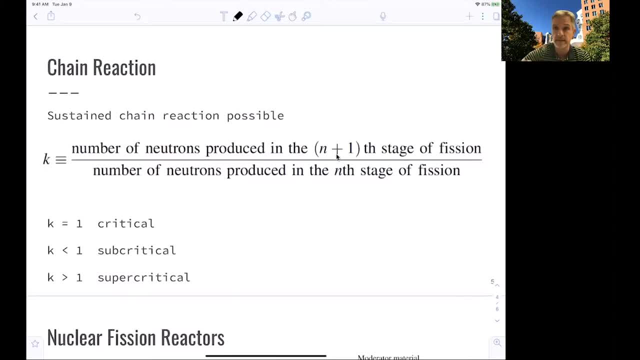 the process is either critical or supercritical, Which means it is able to- because it produces more neutrons than it needs- to continue to have a fission process. it will have or create a chain reaction. If the number is less than 1, the process will die out. 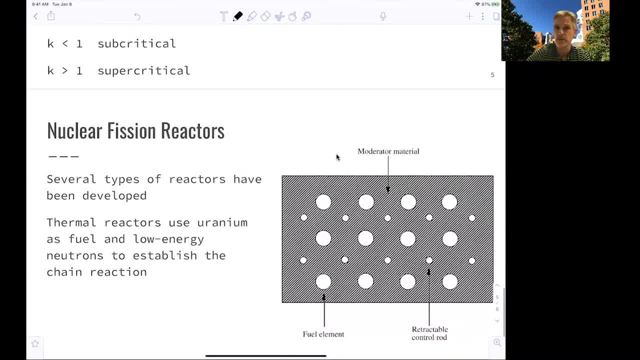 And this is exactly what's used in nuclear fission reactors. There is several types of reactors. The example I want to discuss here very briefly is the one of a thermal reactor which uses uranium as fuel and low energy neutrons to establish the chain reaction as we just discussed. 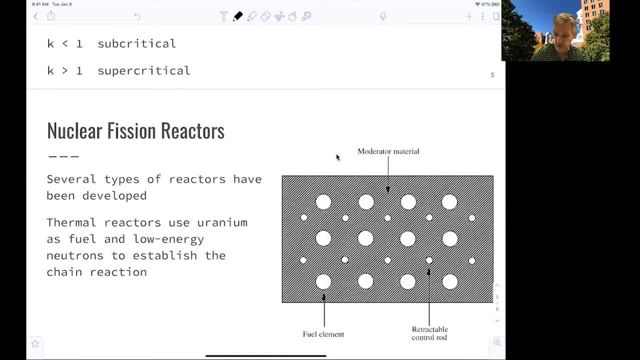 And so this is a sketch here, And the sketch has three different elements. The first one is a fuel element. The fuel element can be naturally occurring uranium, And then we have a moderator material, And the purpose of the moderator material is to generate a chain reaction.